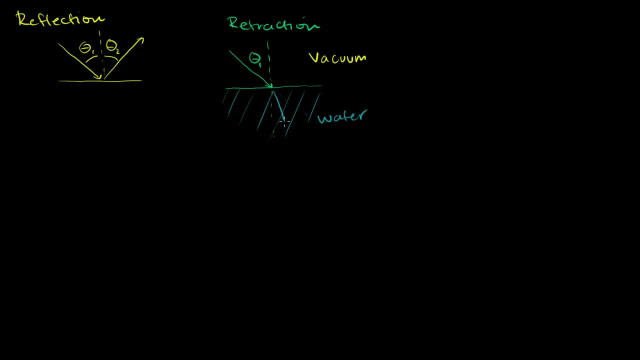 Instead of continuing to go in that same direction, it's going to bend a little bit. It's going to go down in that direction, just like that. And this angle right here, theta 2, is the refraction. That's the refraction angle, or angle of refraction. 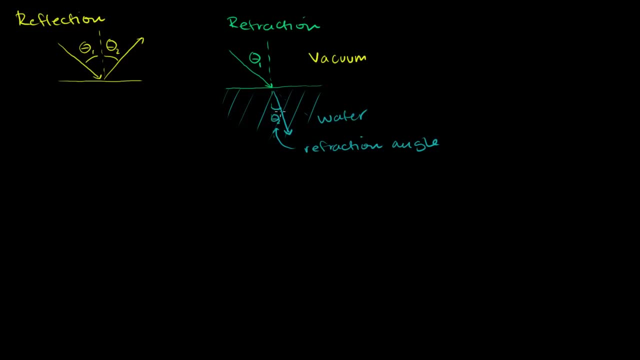 This is the incident angle, or angle of incidence, And this is the refraction angle, once again against that perpendicular, And before I give you the actual equation of how these two things relate and how they're related to the speed of light, 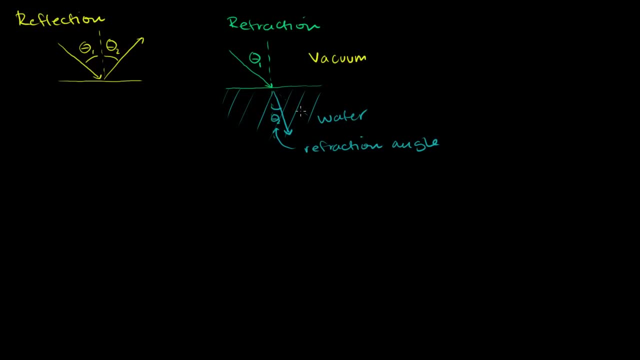 in these two media and just remember once again: you're never going to have vacuum against water. The water would evaporate because there's no pressure on it and all of that type of thing. But before I go into the math of actually how, 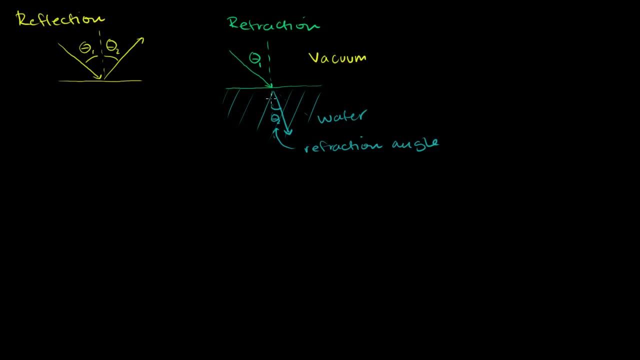 to figure out these angles relative to the velocities of light in the different media. I want to give you an intuitive understanding of not why it bends, because I'm not telling you actually how light works. This is really more of an observed property And light as we'll learn as we do more and more videos about it. 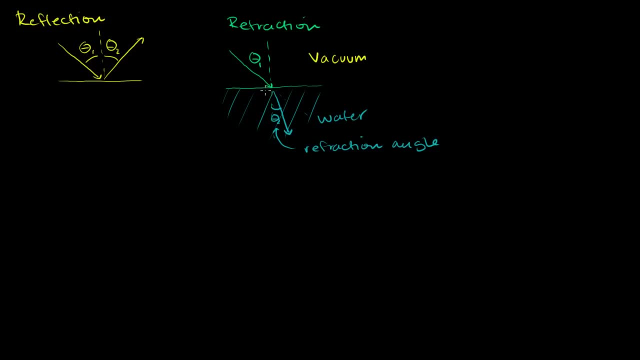 can get pretty confusing. Sometimes you want to treat it as a ray, Sometimes you want to treat it as a wave, Sometimes you want to treat it as a photon, But when you think about refraction, I actually like to think of it as kind of a bit of a vehicle. 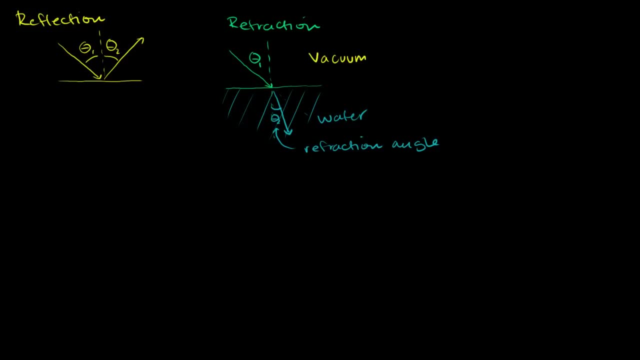 And to imagine that, let's imagine that I had a car, So let me draw a car. So we're looking at the top of the car, So this is the passenger compartment And it has four wheels on the car And we're looking at it from above. 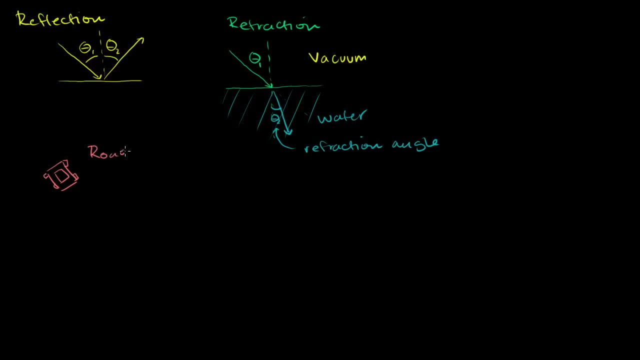 And let's say it's traveling on a road, The tires can get good traction, The car can move pretty efficiently And it's about to reach an interface where the road ends And it will have to travel on mud. Now, on mud, obviously a tire's traction. 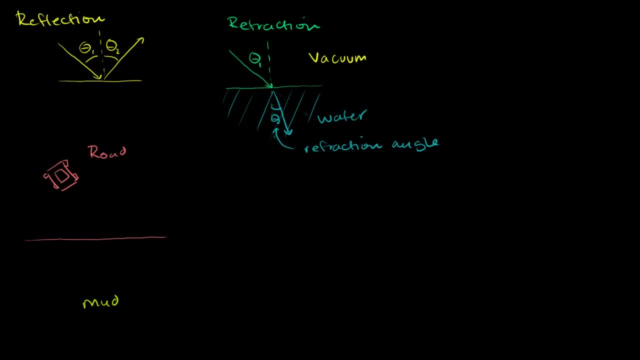 will not be as good. The car will not be able to travel as fast. So what's going to happen? Assuming that the steering wheel isn't telling it to turn or anything, the car would just go straight in this direction. But what happens right when 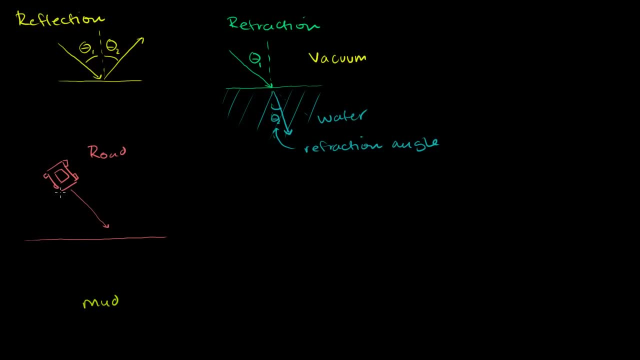 Which wheels are going to reach the mud first? Well, this wheel right here is going to reach the mud first. So what's going to happen? There's going to be some point in time where the car is right over here, Where these wheels are still on the road. 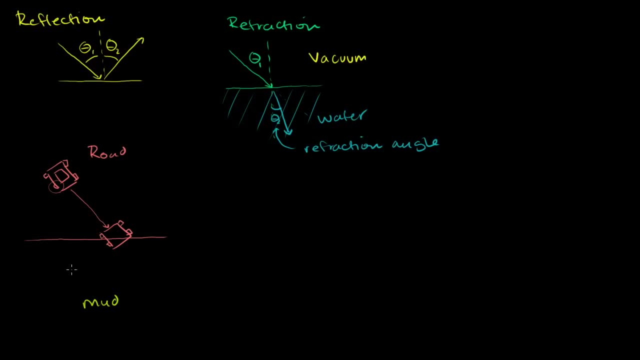 this wheel is in the mud And that wheel is about to reach the mud. Now, in this situation, what would the car do? And assuming that the engine is revving and the wheels are turning at the exact same speed at the entire point of this? 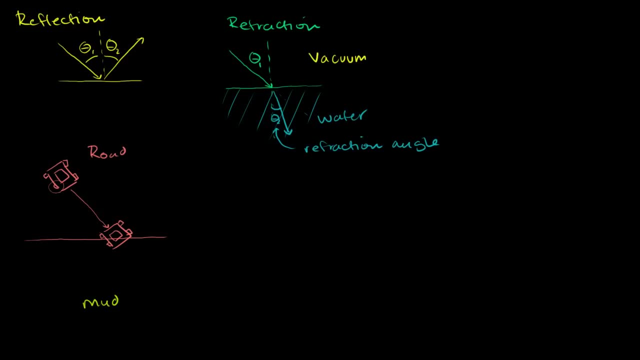 The entire time of the simulation. Well, all of a sudden, as soon as this wheel hits the medium, it's going to slow down. This is going to slow down, But these guys are still on the road, So they're still going to be faster. 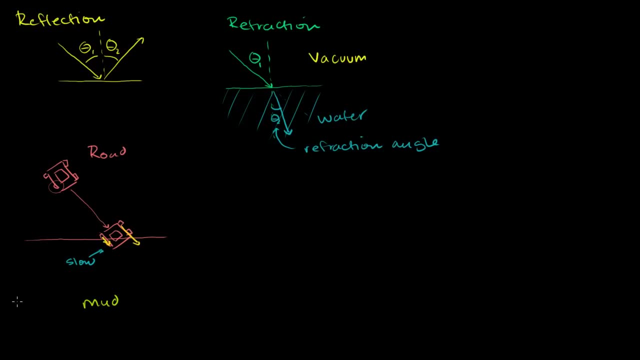 So the right side of the car is going to move faster than the left side of the car. So what's that going to happen? I mean, you see this all the time: If the right side of you is moving faster than the left side of you, you're going to turn. 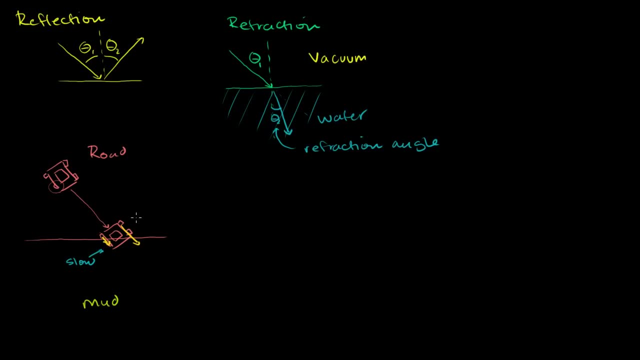 And that's exactly what's going to happen to the car. The car is going to turn, It's going to turn in that direction, And so, once it gets to the medium, it'll now travel, It'll now turn from the point of view, from the car. 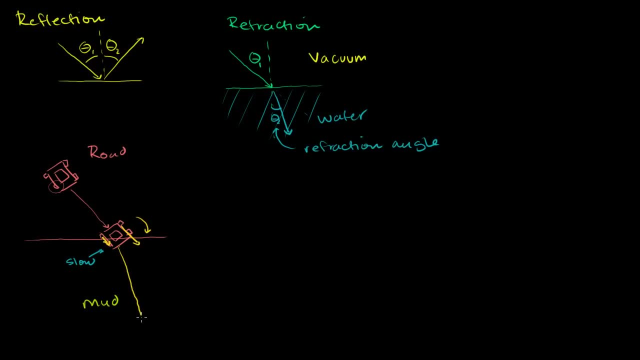 It's turning to the right, But it'll now travel in this direction. It will be turned when it gets to that interface. Now, obviously, light doesn't have wheels and it doesn't deal with mud, But it's the same general idea. 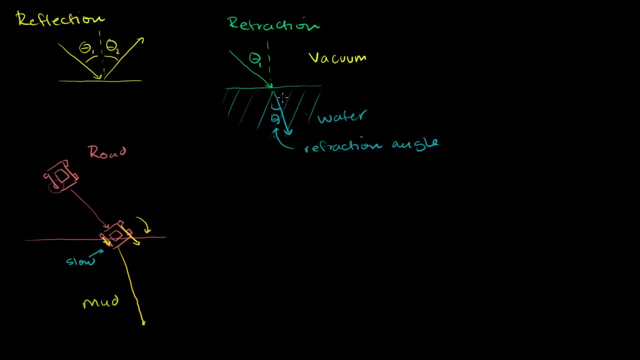 When I'm traveling from a faster medium to a slower medium, you can kind of imagine the wheels on that light on this side of it, closer to the vertical, hit the medium first, slow down. So the light turns to the right. 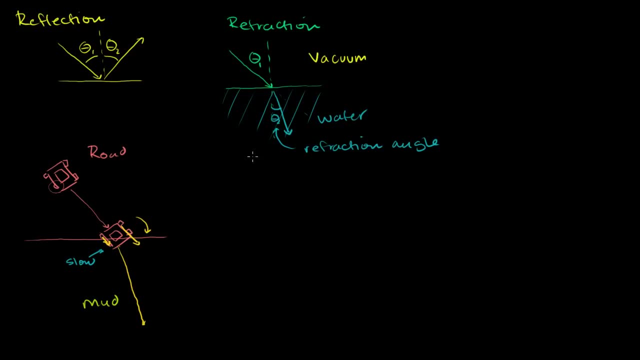 If you're going the other way, if I had light coming out of the slow medium. so let's imagine it this way: Let's have light coming out of the slow medium And if we use the car analogy in this situation, the left side of the car is going to. 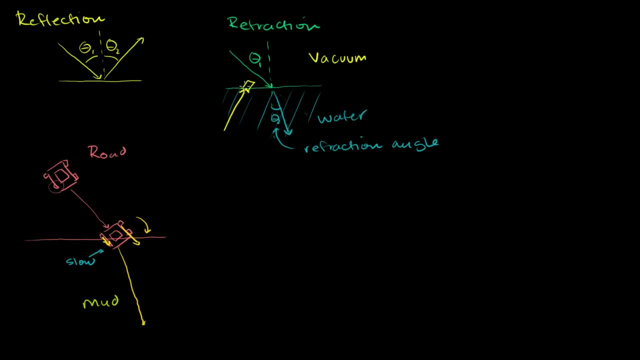 so if the car is right over here, the left side of the car is going to come out first, So it's going to move faster now. So the car is going to turn. It's going to turn to the right, just like that. 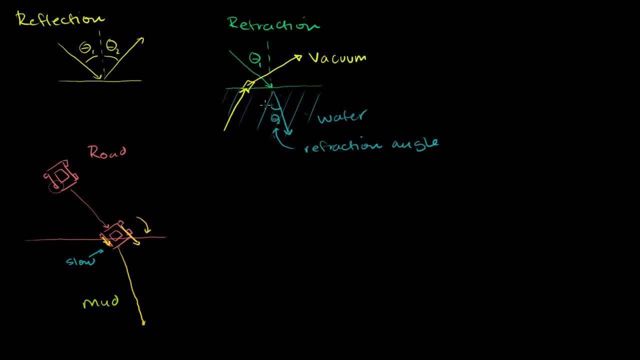 So hopefully this gives you a gut sense of just how to figure out which direction the light's going to bend. if you just wanted an intuitive sense And to get to the next level, there's actually something called Snell's Law, And all this is saying is that this angle. 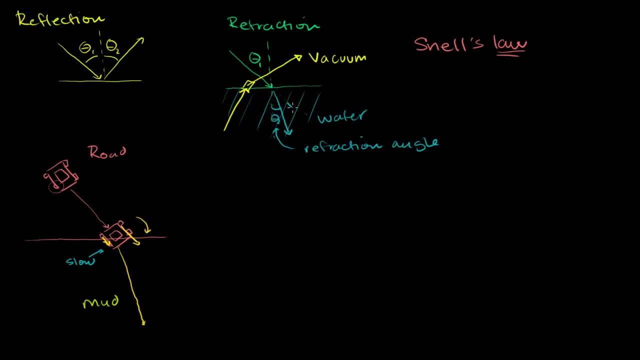 so let me write it down here. So let's say that this velocity right here is velocity 2.. This velocity up here was velocity 1, going back to the original. Actually, let me draw another diagram just to clean it up, And also I have that vacuum water interface example. 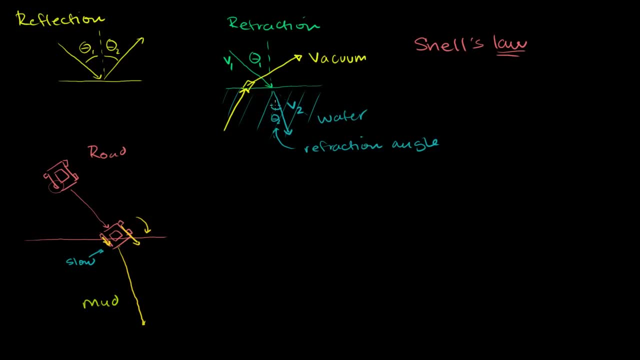 I'm not enjoying it just because it's a very unnatural interface to actually have in nature. So maybe it's vacuum and glass. That's something that actually would exist. So let's say we're doing that, So this isn't water. 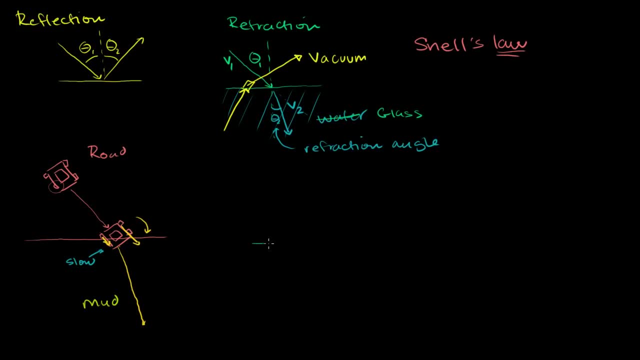 This is glass. This is glass, So let me redraw it And I'll draw the angles bigger. So let me draw a perpendicular, And so I have our incident ray. So in the vacuum it's traveling at v1. And in the case of a vacuum, it's actually. 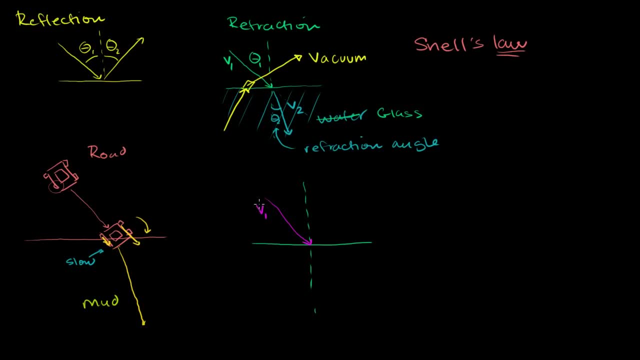 going at the speed of light, or speed of light in a vacuum, which is c or 300,000 kilometers per second, or 300 million meters per second. Let me write that So: c is the speed of light in a vacuum. 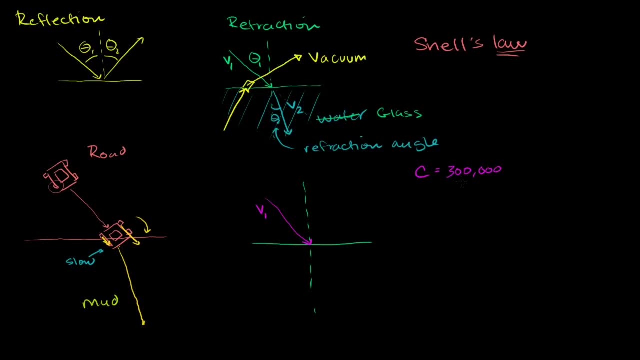 And that is equal to 300.. It's not exactly 300.. I'm not going to significant digits. It's true to three significant digits: 300 million meters per second. This is light in a vacuum And I don't mean the thing that you. 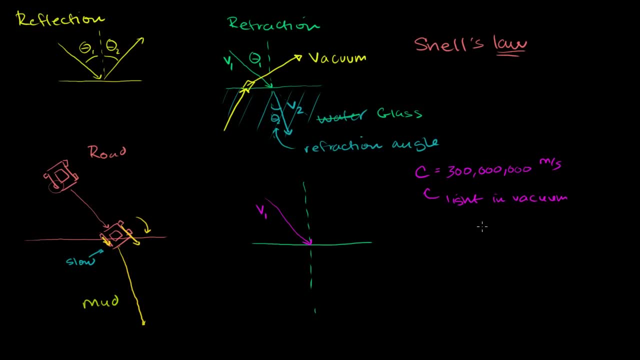 use to clean your carpet. with I mean an area of space that has nothing in it: No air, no gas, no molecules, nothing in it. That is a pure vacuum. And that's how fast light will travel. Now it's traveling really fast there. 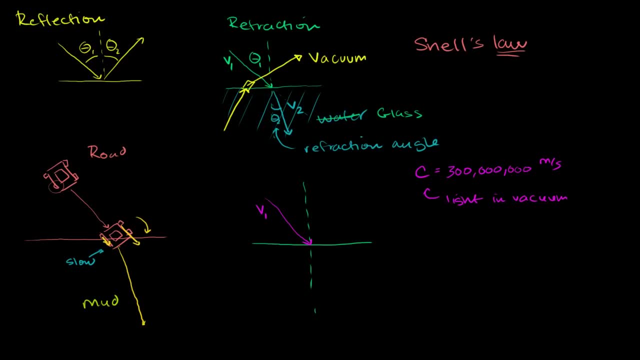 And let's say that this is, and this applies to any two medium. But let's say this is, let's say it gets to glass here And in glass it travels. It travels slower And we know, for example, this side of the car. 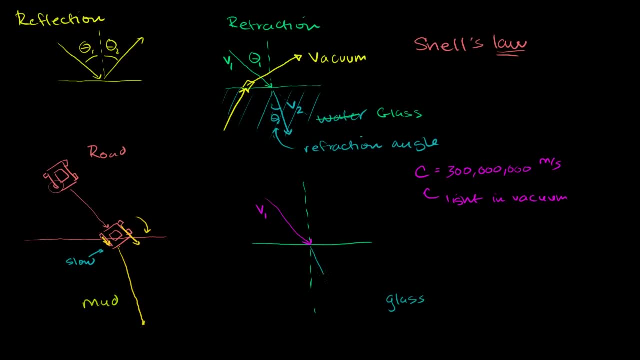 is going to get to the slow medium first. So it's going to turn in this direction. So it's going to go like this And we call this v2.. And maybe I'll draw it If you wanted to view these as vectors. 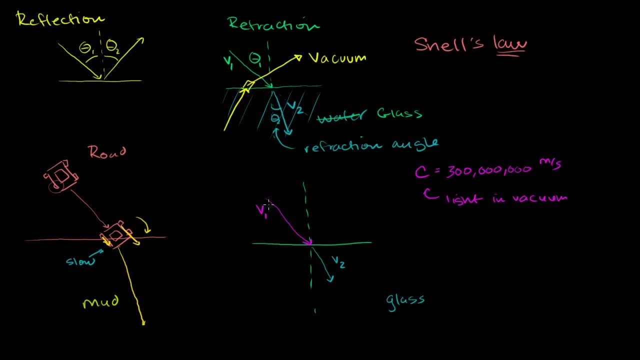 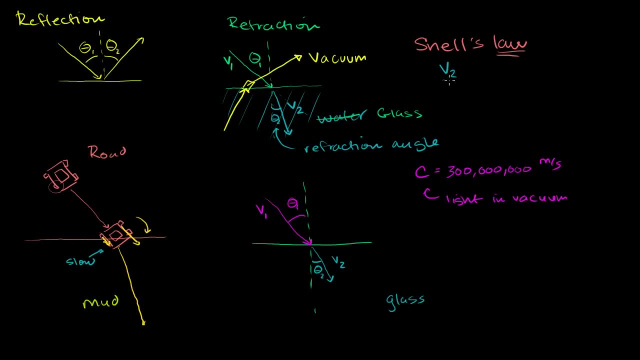 Snell's law just tells us that the ratio between v2 and the sine- remember SOHCAHTOA, basic trig function- and the sine of the angle of refraction is going to be equal to the ratio of v1, and the sine of the angle of incidence, sine of theta 1.. 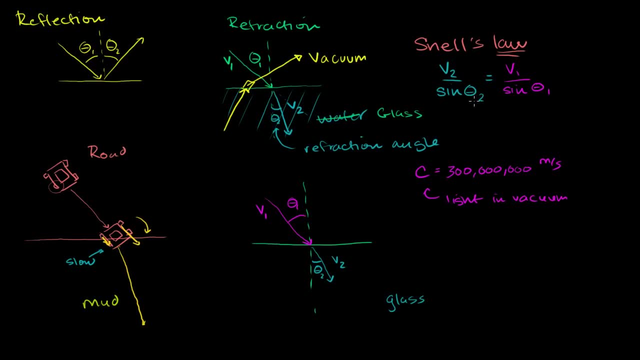 Now, if this looks confusing at all, we're going to apply it a bunch in the next couple of videos, But I want to show you Also that there's many, many ways to view Snell's law. You may or may not be familiar with the idea. 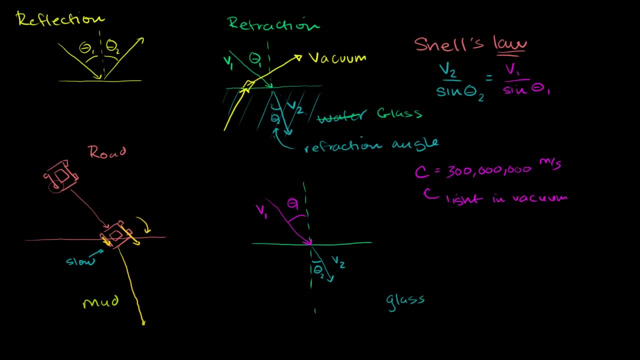 of an index of a refraction. So let me write that down: Index of a refraction Index or a fraction index, And it's defined, And it's defined for any material. There's an index of a refraction for a vacuum, for air. 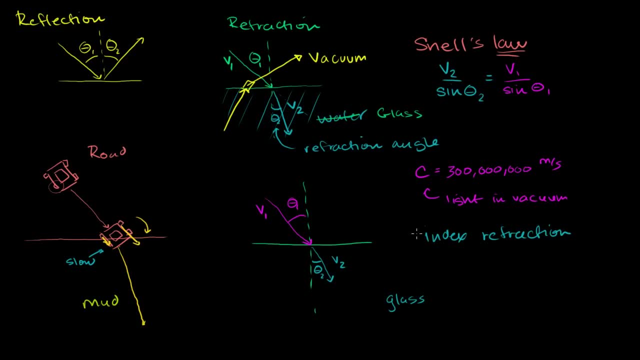 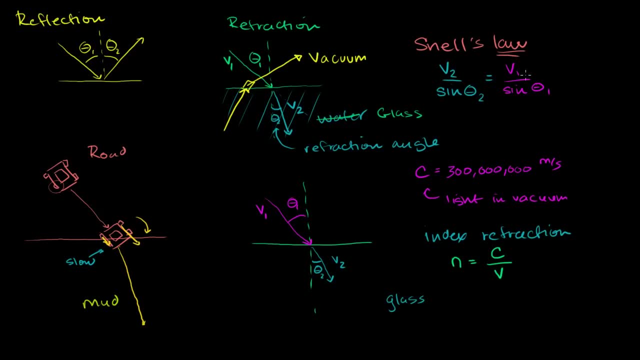 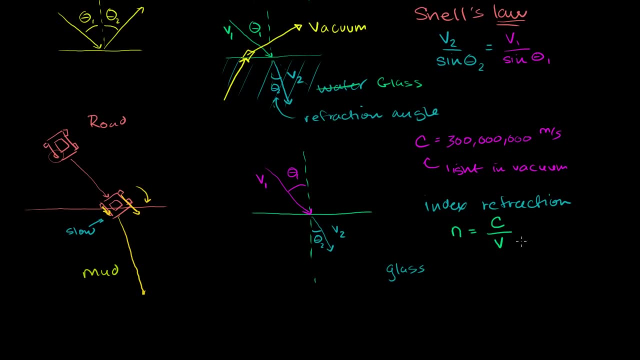 So in our example right here we could rewrite this in terms of index of refraction. Let me do that actually just because that's sometimes a more typical way of viewing Snell's law. So I could solve for v here. One thing I can do is just if n is equal to c divided by v. 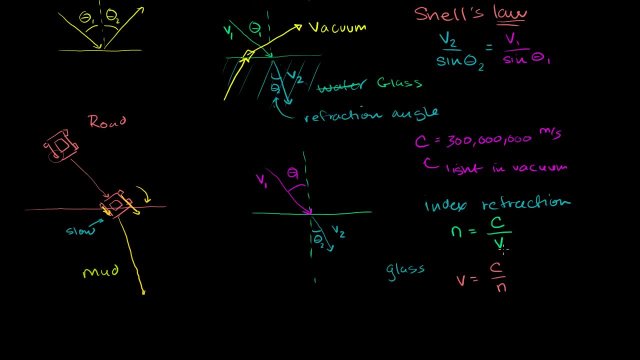 then v is going to be equal to c divided by n, And I can multiply both sides by v. if you don't see how I got there, The intermediary step is: multiply both sides. times v, You get v. times n is equal to c. 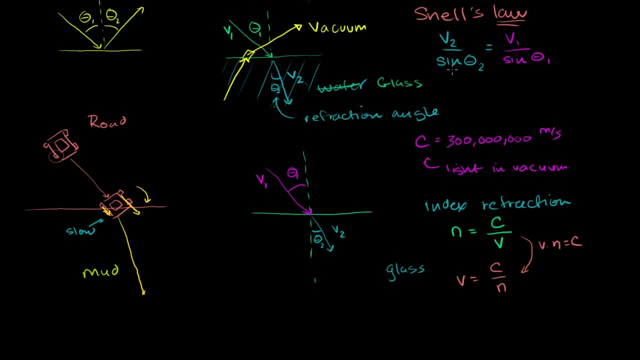 And then you divide both sides by n, You get v is equal to c over n. So I can rewrite Snell's law over here, as instead of having v2 there, I could write. instead of writing v2 there, I could write the speed of light. 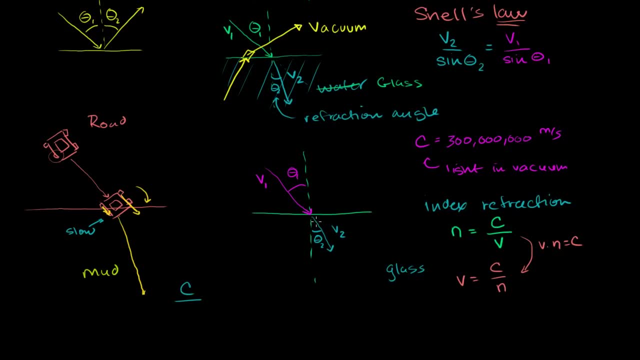 Speed of light divided by the refraction index for this material right here, So I'll call that n2.. This is material 2. right over there That's the same thing as v2. over the sine of theta, 2 is equal to v1, is the same thing as c divided by n1. 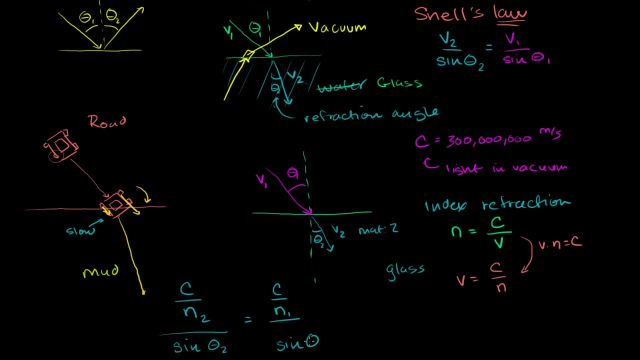 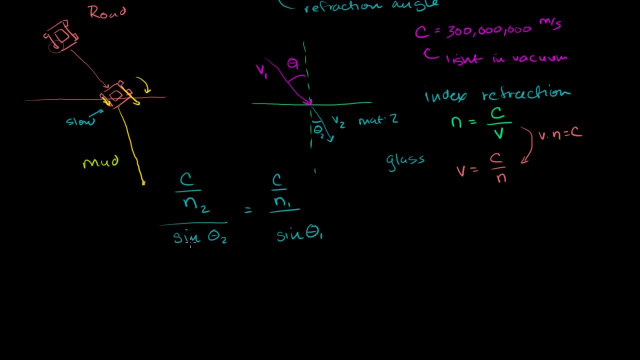 over sine of theta 1.. And then we could do a little bit of simplification here. We can multiply both sides of this equation. Well, let's do a couple of things. Actually, the simplest thing to do would actually take the reciprocal of both sides. 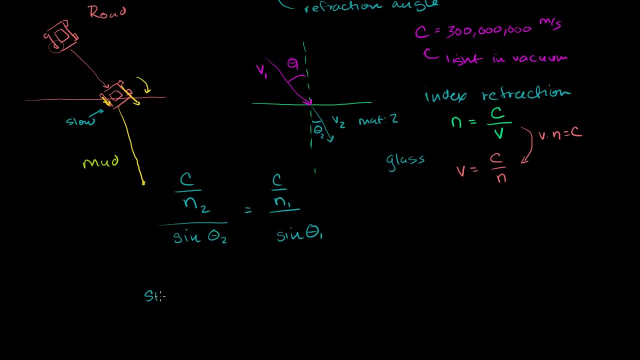 So let me just do that. So if we take the reciprocal of both sides of this, you get: sine of theta 2 over c? n2 is equal to sine of theta 1.. So the reciprocal of theta 2 over c? n1 is equal to sine of theta 1.. 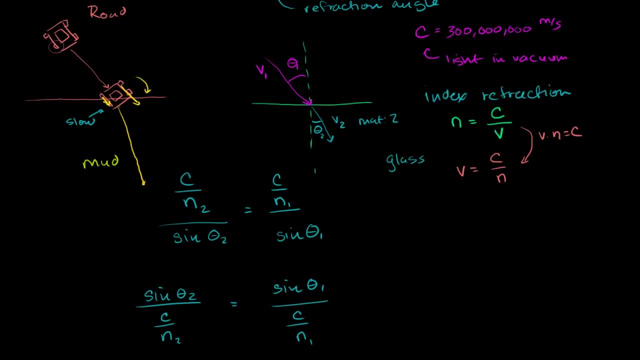 And now let's multiply the numerator and denominator of this left side by n2.. So if we multiply n2 over n2, we're not changing it. This is really just going to be 1.. But this guy and this guy are going to cancel out. 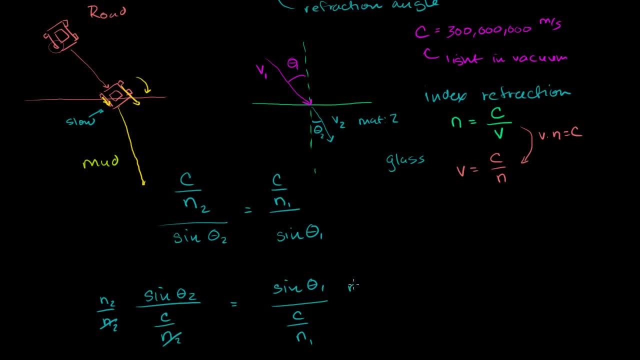 And let's do the same thing over here: Multiply the numerator and the denominator by n1.. So n1 over n1.. That guy and that guy are going to cancel out, And so we get n2 over n2.. And this guy I'm going to cancel out. 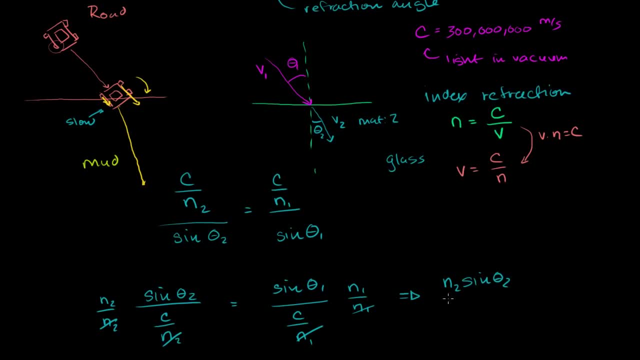 And so we get n2 over n2.. And so we get n2 over n2.. And so we get n2 over n1.. And so we get n2 over n1.. sine of theta 2 over c is equal to n1. sine of theta 1 over c. 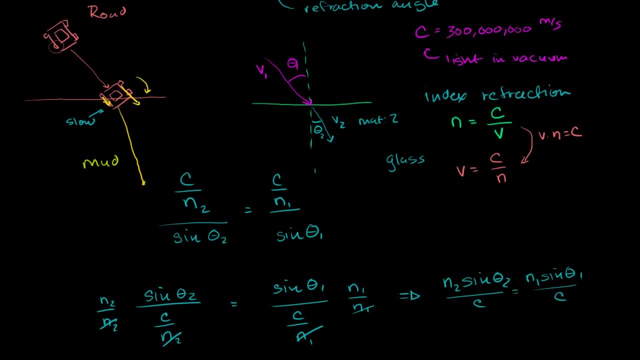 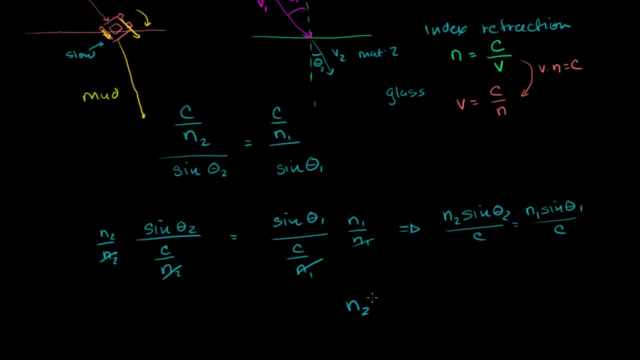 And now we can just multiply both sides of this equation by c and we get the form of Snell's law that some books will show you, which is the refraction index for the slower medium or for the second medium, the one that 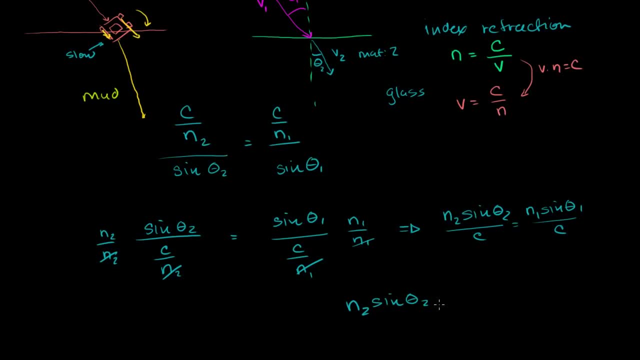 we're entering times. the sine of the index refraction is equal to the refraction index for the first medium times, the sine of the angle of incidence, the incident angle. So this is another version right here. This is another version right there of Snell's law. 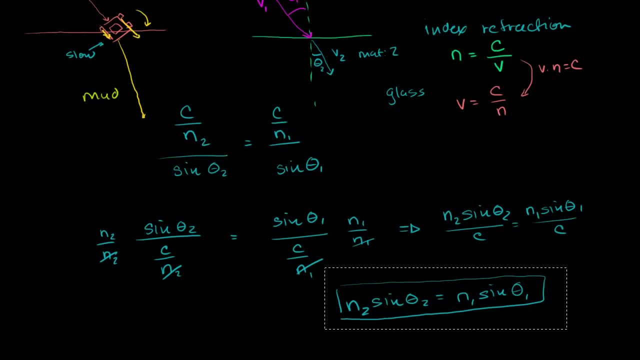 Let me copy and paste that. And if this is confusing to you- and I'm guessing that it might be, because, especially if this is the first time that you see it- we're going to apply this in a bunch of videos in the next few videos. 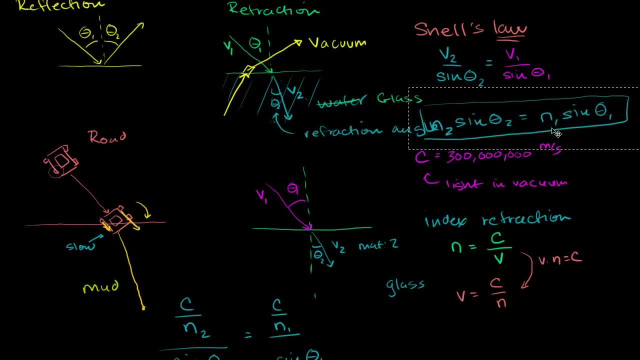 But I really just want to make sure you're comfortable with it. so these are both equivalent forms of Snell's law. One deals with the velocities, directly deals with the velocities right over here, the ratio of the velocity to the sine of the incident, or refraction angle.